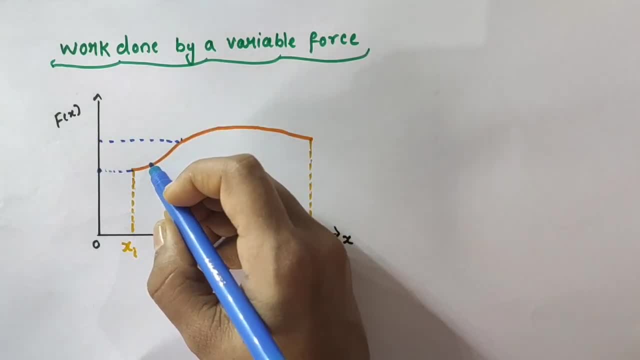 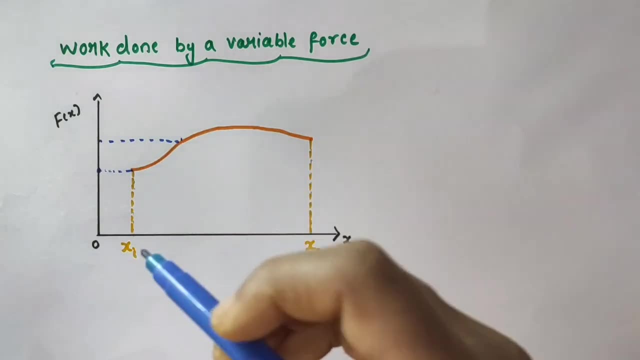 force varies. now, Then somewhere here the force will be different. Alright, That is. force changes from point to point. That is here we have a varying force. Okay, Now let xi be the initial position of that object and xf be the final position of the object. Then what about the? 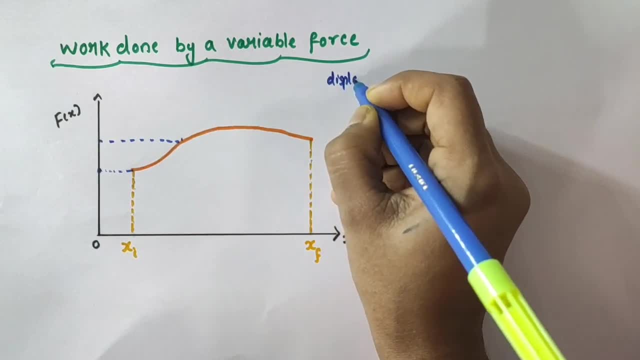 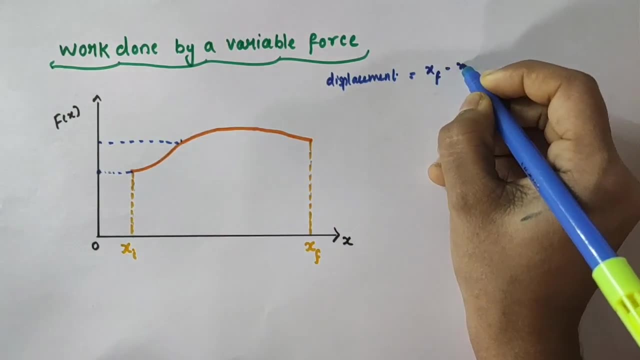 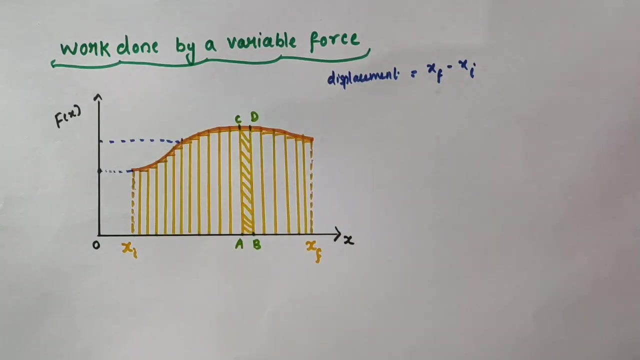 displacement. The total displacement will be what? The total displacement, actually the displacement of that object, when we consider the whole motion of that body, will be equal to what The final position minus initial position, That is, xf minus xi. Okay, Now, here you see I have just divided. 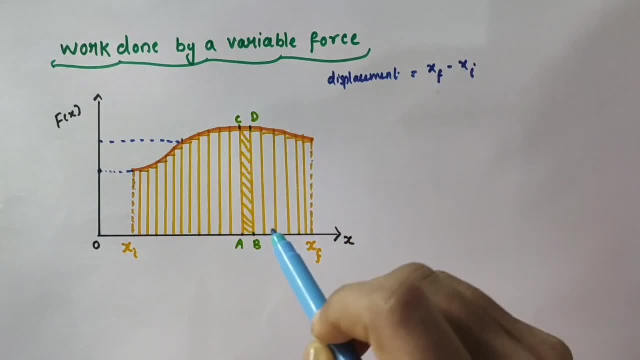 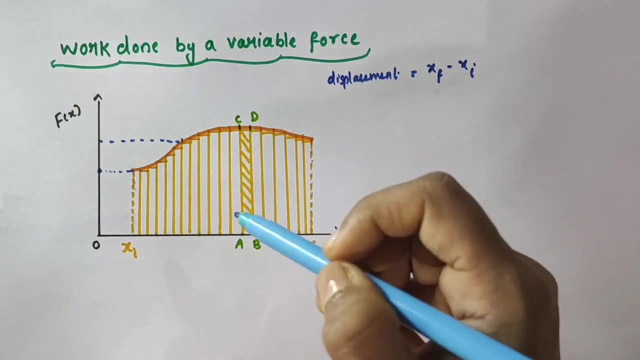 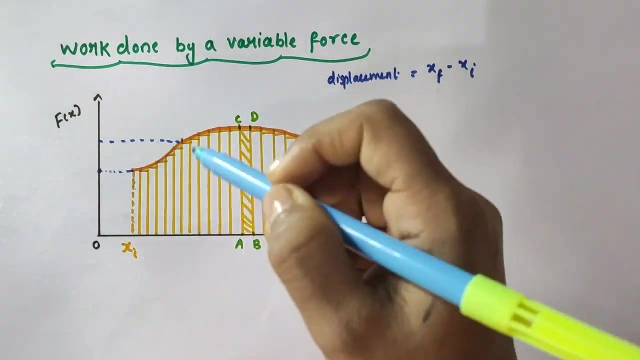 the whole area under this graph into small, small, small successive rectangular areas. Okay, And I am considering a small area. This must be, I mean all must be having. I mean we just want to divide them into small, small areas, That is all Okay. Now here, just consider a small area. 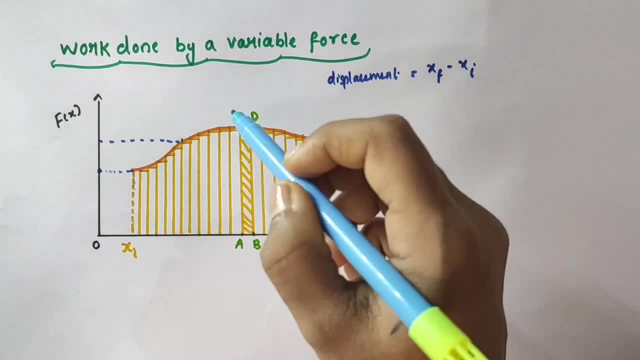 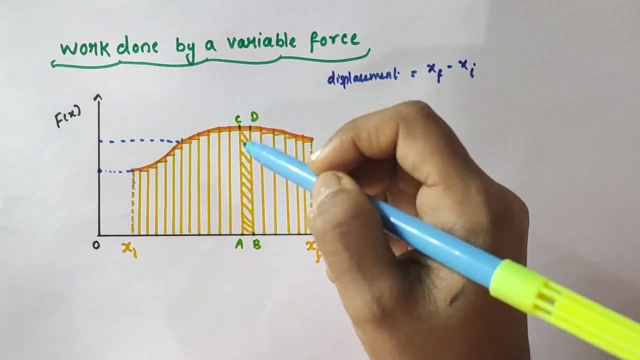 element. Let this point be A, this is B, and this is C and this is D. So here you see, I am just finding out the area of the small rectangular area: element A, B, D, C or A C, D, B, like that. 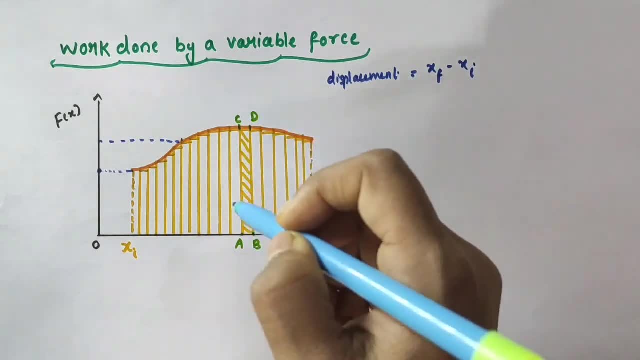 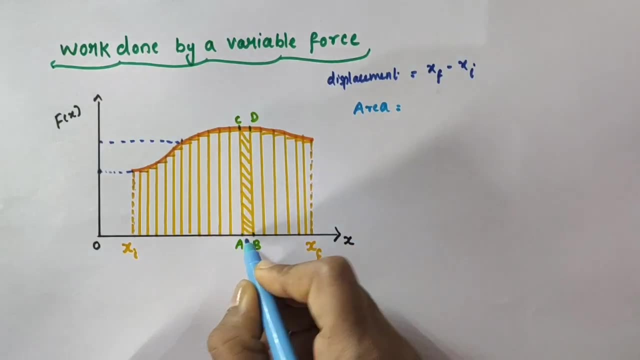 Okay, Now how can we find out the area of this rectangular element? actually, Area is equal to what? Length into breadth? no, So I am considering we can write it as A B into B D. no, Okay One. 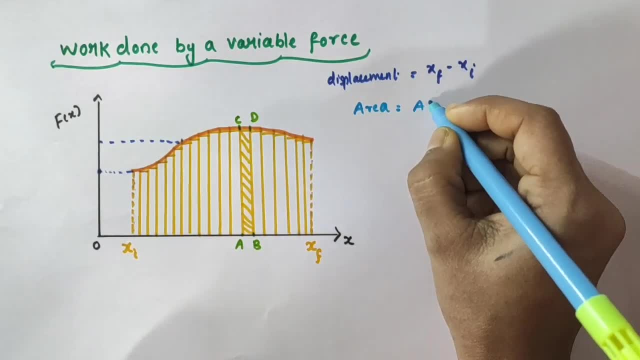 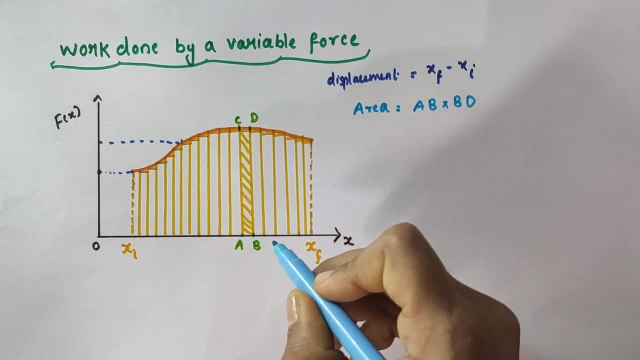 side into the other side will give you the area. no, Okay, So area is equal to A B into B D. Okay, See, A B is actually the difference in these two positions, A and B. no, So we can. 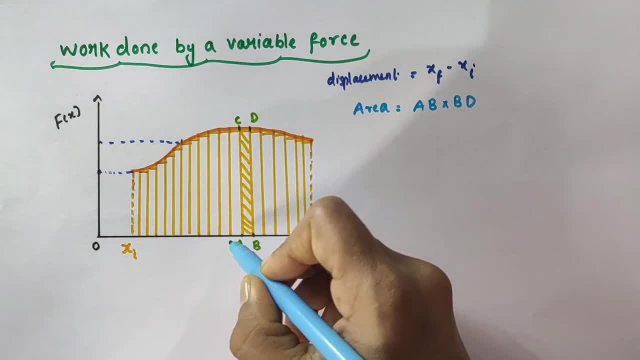 consider A, B as the displacement, no Final position minus initial position. So we can position like that: Okay, And here the displacement we have considered a very small area element, So this distance is very less Okay. So the displacement A- B that will be. 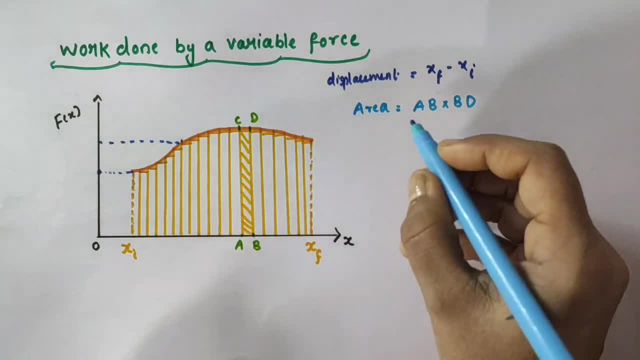 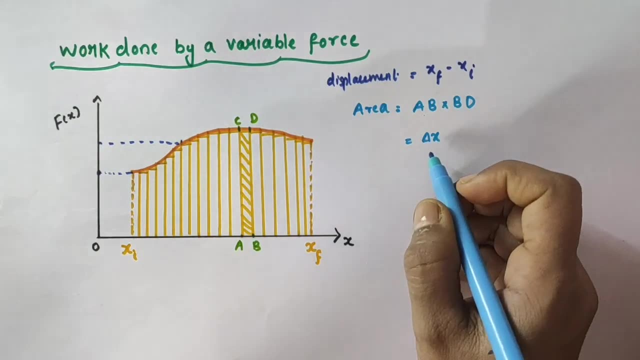 very small. no, So I am considering: I am representing it with delta x. Okay, I am taking A B as the displacement which is very small. So I am representing the displacement as delta x. Okay, Now what about B D? B D: it is the side of this rectangle which is parallel to the force. 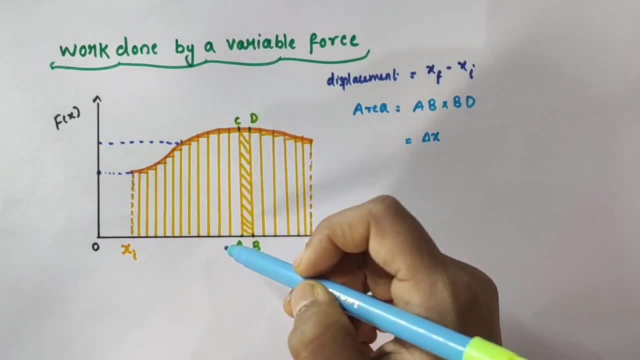 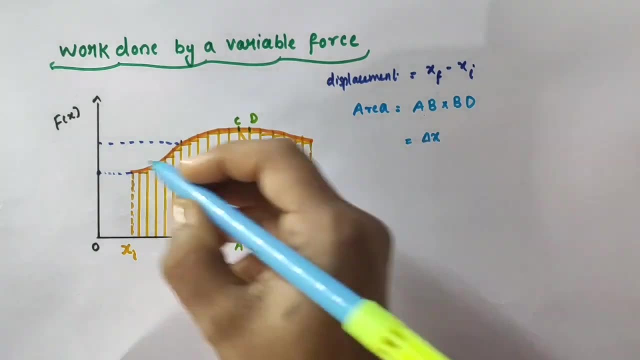 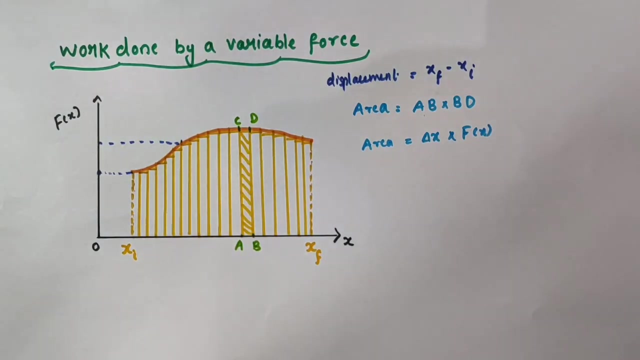 force. Okay, If the displacement delta x is very small, we can take this force F of x as approximately a constant. Okay, So I am taking B D as F of x. So we are getting area as delta x into F of x. Okay, Now this is actually what force into displacement? no, Okay, This. 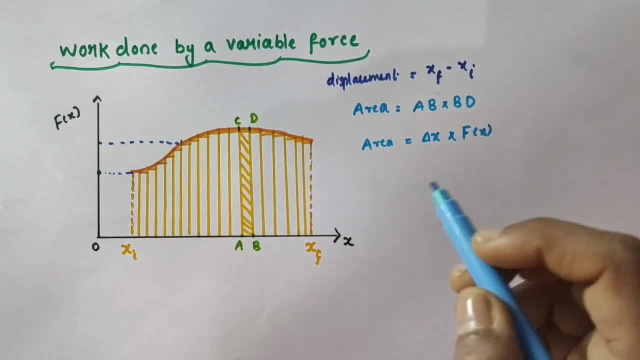 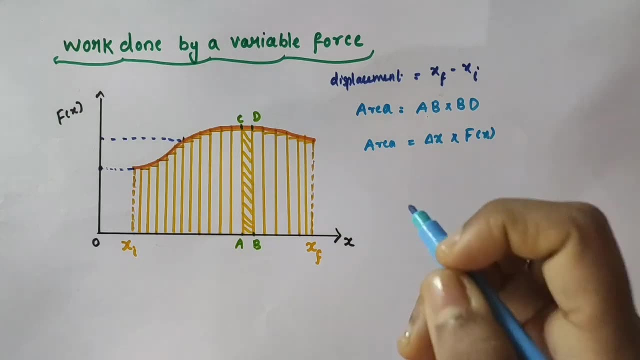 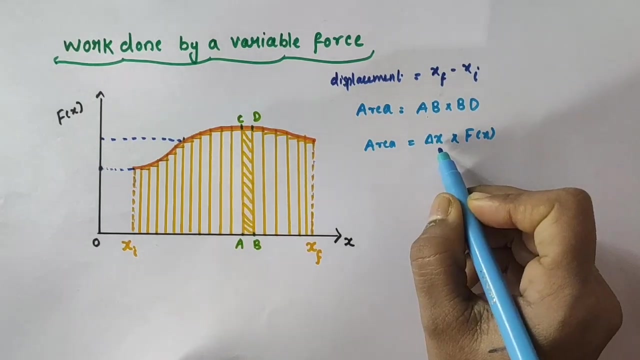 is force and this is displacement. What is force into displacement? It is the work done. no, Since the displacement, the work done will also be small. So I am representing this area. that is equal to the work done. no, Because force into displacement. Since the displacement is small, the work done. 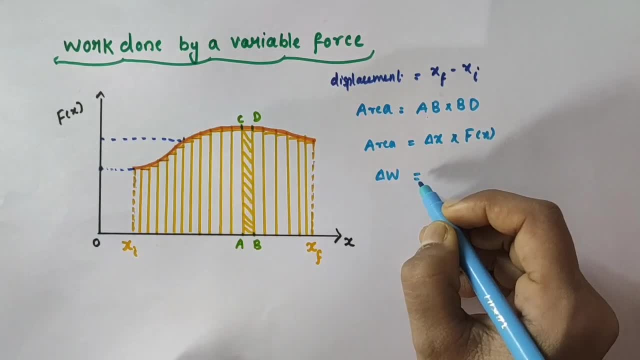 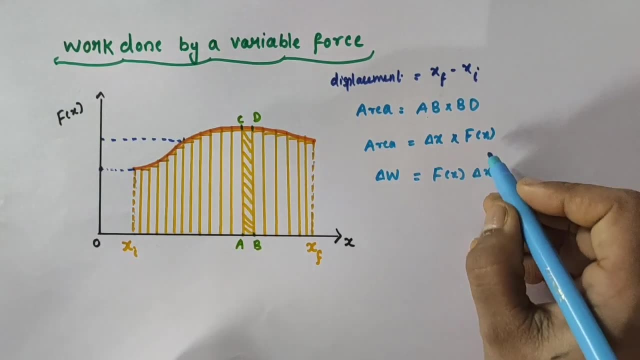 is also small, So I am representing that work done as delta w. Okay, So we can write delta w is equal to F of x into delta x. Okay, We can write delta w is equal to F of x into delta x. 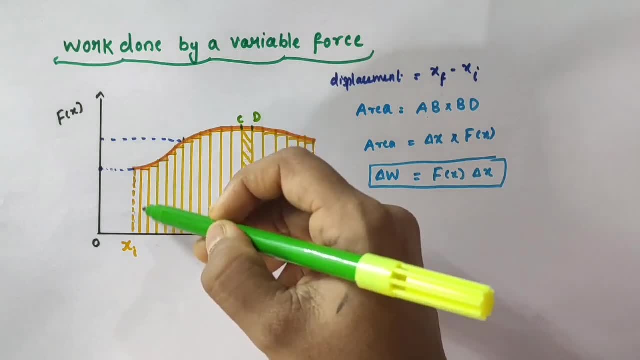 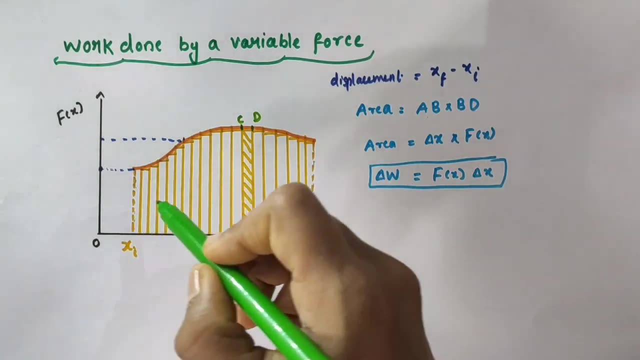 Similarly, we can consider this small area element. we can consider this small area element, Okay, And we can find out the corresponding work done. Okay, You can consider each and every small, small, small area elements and you can find out the respective work done. 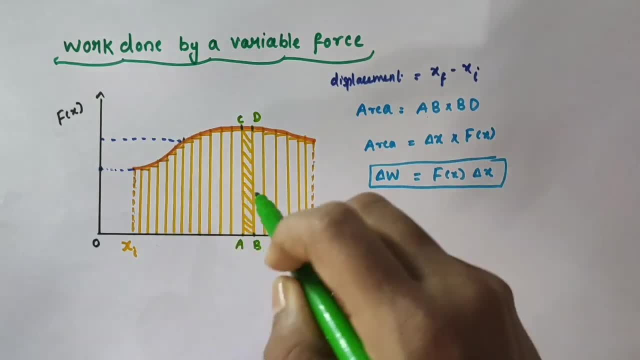 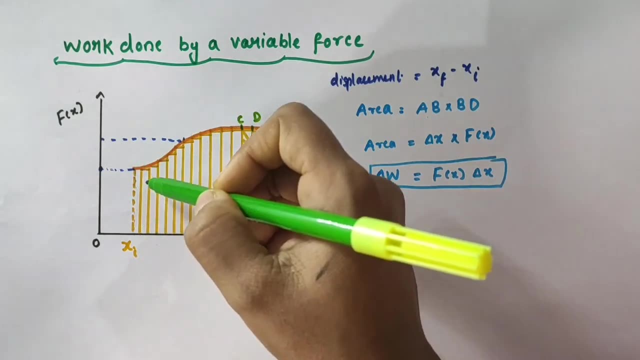 All right, And by adding all those, you will get the total work done. Okay, You can find out the work done corresponding to this. considering this area element. You can consider this area element and you can find out the corresponding work done. You can consider this area element. you can find. 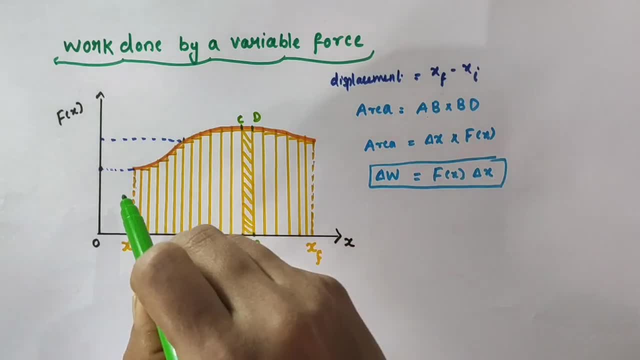 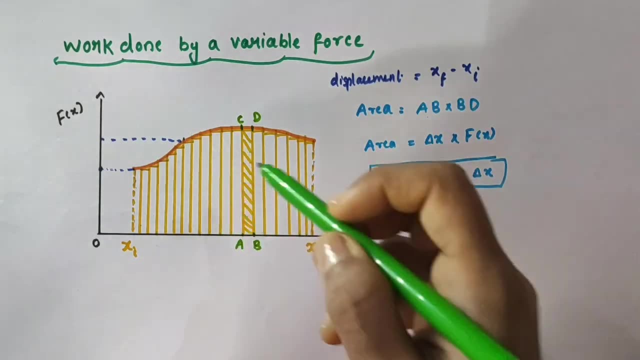 out the corresponding work done, Such that you can- I mean, like that you can- consider all the area elements and you can find out the respective work done And you can add all those work done. you will get the total work done. Okay, That is the total work. 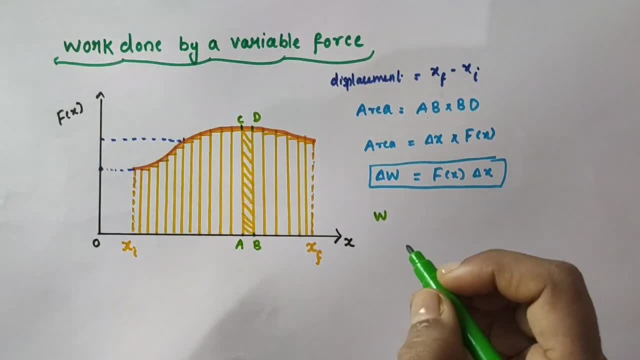 done. w. Okay, Total work done. so w Total work done can be written as what: Summation xi to xf, F of x into delta x. That is summation over xi to xf, F of x into delta x. Why summation? 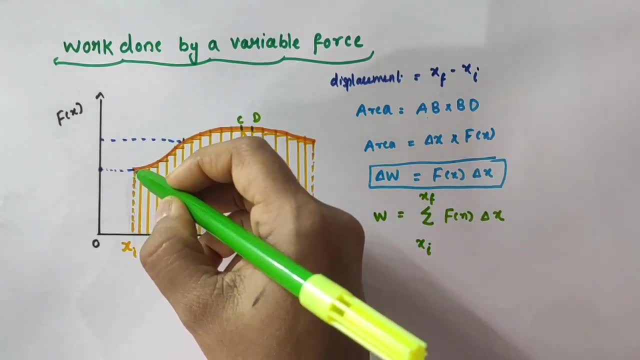 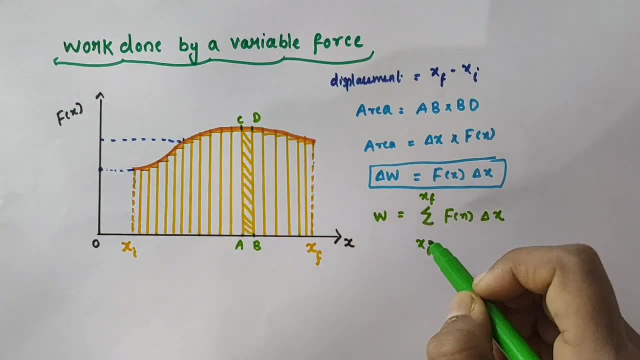 over xi to xf. That is summation means we are adding: We want to find out the corresponding work done by considering each area rectangular element here. Then we want to add: That is why summation. Then why summation over xi to xf? Because we are finding out the total work done. 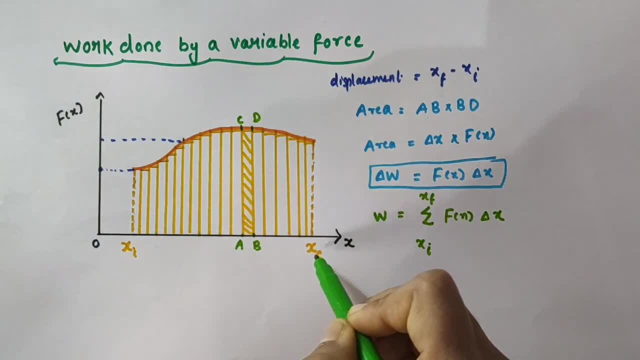 So we have to take the sum from here to here. Okay, That is, the summation is from the initial position to the final position: xf. Okay, That is why xi to xf. All right Now, if the displacement allowed to approach 0,, that is, when delta x tends to 0,, we can write this expression as w is equal. 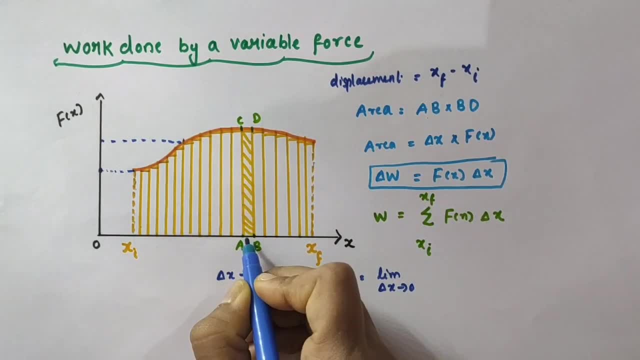 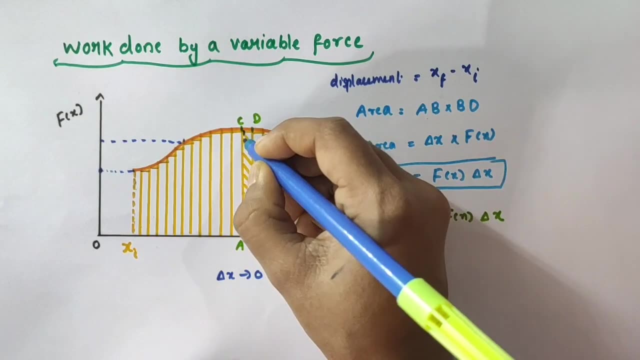 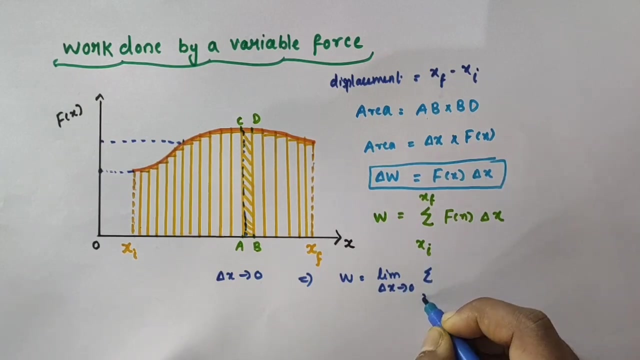 to limit delta x tends to 0. That is, we just want to consider very small. I mean a very small rectangular element here. Okay, Very small, That is, the displacement would be very less. That is approximately equal to 0.. All right, Then. limit delta x tends to 0.. Summation xi to xf: F of x into. 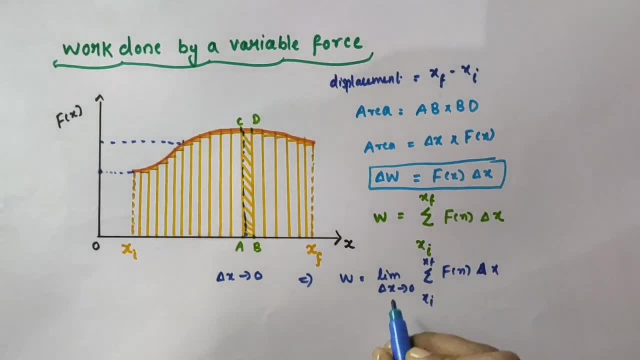 delta x. Okay, Now limit. delta x tends to 0. Summation over xi to xf and delta x, That can be written as: what W is equal to integral xi to xf, Then F of x into dx. Okay, Actually, this equation. 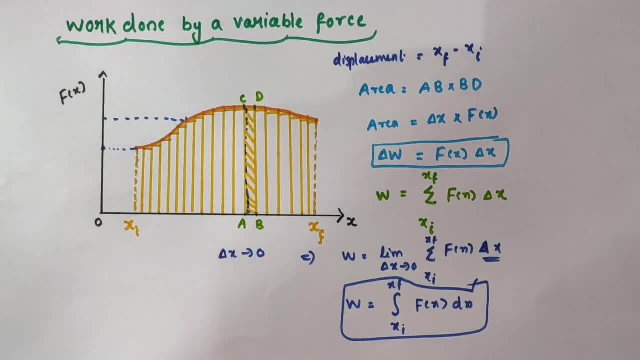 limit, delta x tends to 0.. Summation over xi to xf. F of x into delta x can be written as integral: xi to xf, F of x into dx. Okay, So that is the summation over xi to xf. That is we just want to. 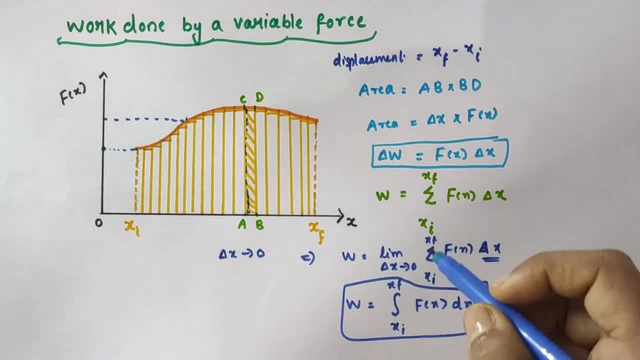 Okay, That is when we take the limit. delta x tends to 0,. this continuous summation, this is the continuous summation or continuously we are adding. So this continuous summation can be replaced by integration. Okay, That is here. actually, limit stands for the limit of the sum when delta x 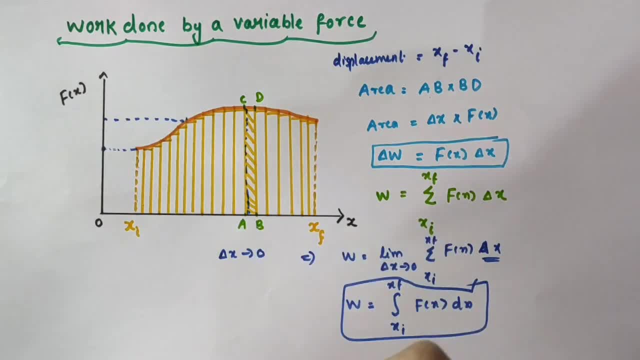 tends to 0. That is when the displacement are allowed to 0.. Okay, When the displacement allowed to approach 0, the number of turns in the sum increases without limit. No, But the sum approaches to a definite value which is equal to the limit of the sum. Okay, So that is when we take the.